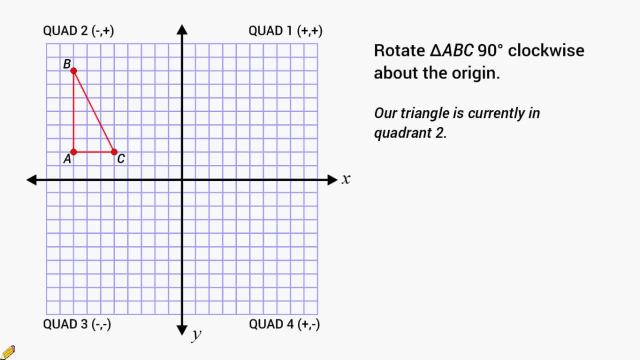 are positive. It is important, with 90 degree rotations, to figure out what the x values and the y values will be in terms of negative and positive. Well, we are going to be rotating our triangle to quadrant number one and in quadrant number one, all of your x values will be positive. 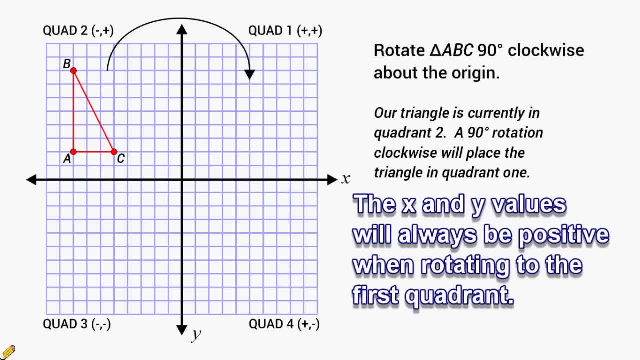 and all your y values will be positive. So one thing we know for sure is that the new location of each of our points will all have positive values because they are being rotated to quadrant number one. So the first thing that we're going to do is 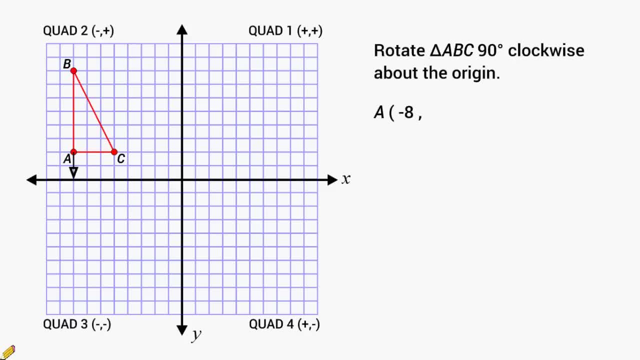 identify the current location of our points. A is located at negative eight positive two, B is located at negative eight, positive eight And C is located at negative five positive two. Okay, now that we have identified the current location of our three points. 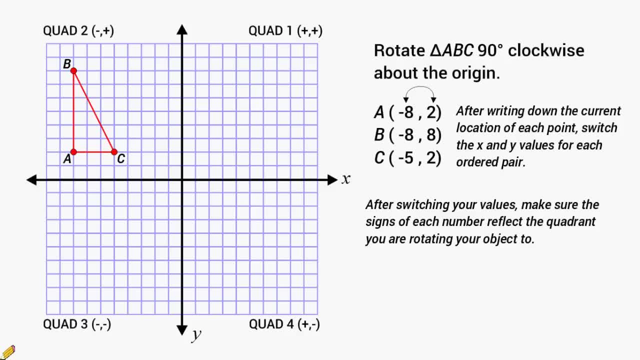 what we're going to do next is switch around the x and the y values, and we're going to start with point A. Now. point A is currently located at negative eight, positive two, And what we have to do is switch around the x and the y values, But for now, let's just ignore whether. 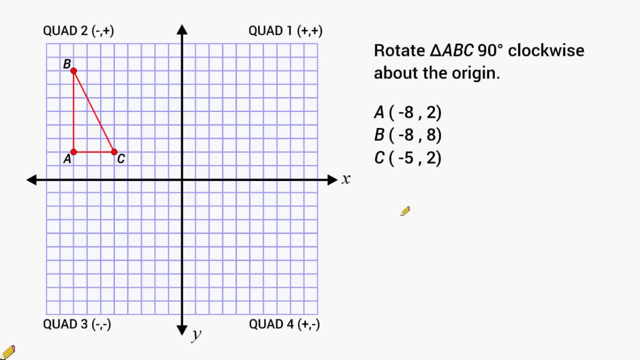 the numbers are negative or positive. Let's just look at the absolute value of the x and the y value. So let's just take eight and two of point A and switch them around and simply write two and eight. Now, because we are rotating our point to quadrant one, we know that all x values as well as all y values in the equation are positive. 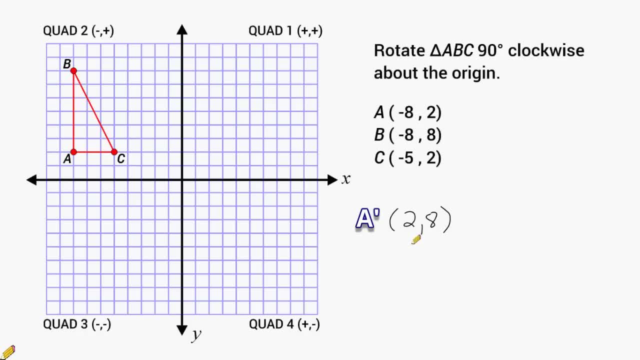 And that quadrant will be positive. So after switching the absolute values of eight and two to be two and eight, we know that both of these values will be positive. Now point B has a current location of negative eight and positive eight And the absolute values are both eight. So even if we switch those, both of them will still be eight. 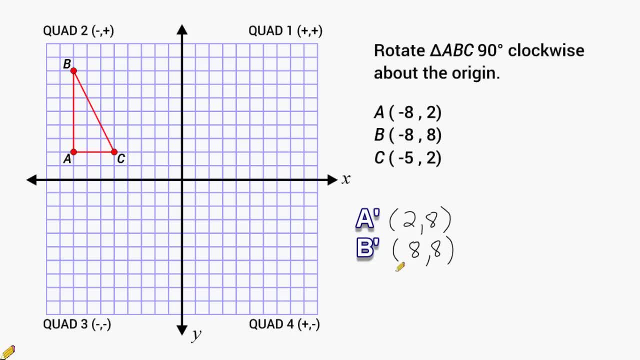 And they will be positive because we are rotating our point to quadrant number one. And for point C we're going to take five and two and switch those around and write two and five And once again both the x and the y values will become positive because they are in quadrant number one. 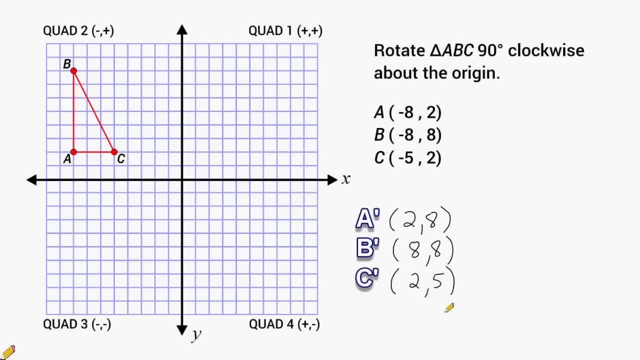 Now that we have the coordinates to where our triangle is going to be rotated to, let's go ahead and plot those points. So point A is going to be at positive two positive eight, And point B is going to be at positive eight, positive eight. 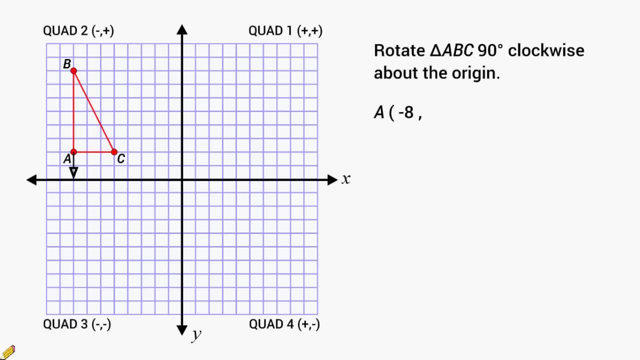 identify the current location of our points. A is located at negative eight positive two, B is located at negative eight, positive eight And C is located at negative five positive two. Okay, now that we have identified the current location of our three points. 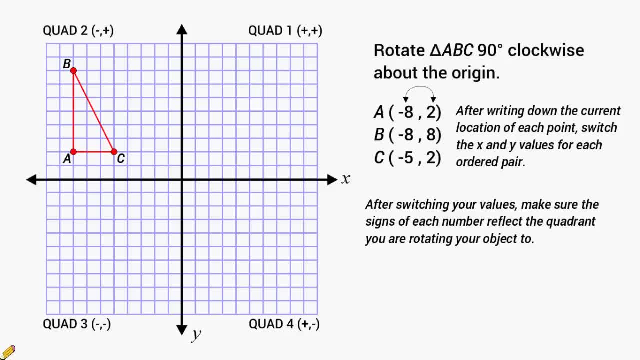 what we're going to do next is switch around the x and the y values. Let's start with point A Now. point A is currently located at negative eight, positive two, And what we have to do is switch around the x and the y values. But for now let's just ignore whether the 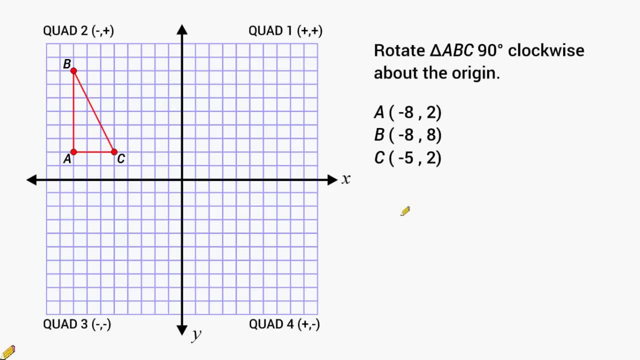 numbers are negative or positive. Let's just look at the absolute value of the x and the y value. So let's just take eight and two of point A and switch them around and simply write two and eight. Now, because we are rotating our point to quadrant 1, we know that all x values as well. 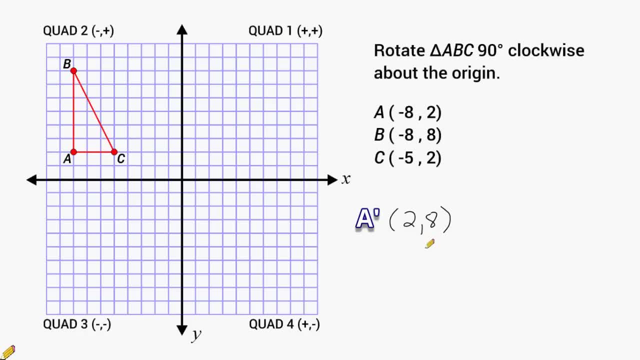 as all y values in that quadrant will be positive. So after switching the absolute values of 8 and 2 to be 2 and 8, we know that both of these values will be positive. Now point B has a current location of negative 8 and positive 8 and the absolute values are: 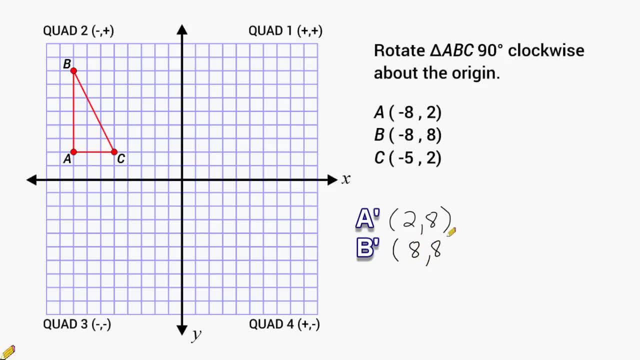 both 8, so even if we switch those, both of them will still be 8 and they will be positive because we are rotating our point to quadrant number 1.. And for point C, we're going to take 5 and 2 and switch those around and write 2 and 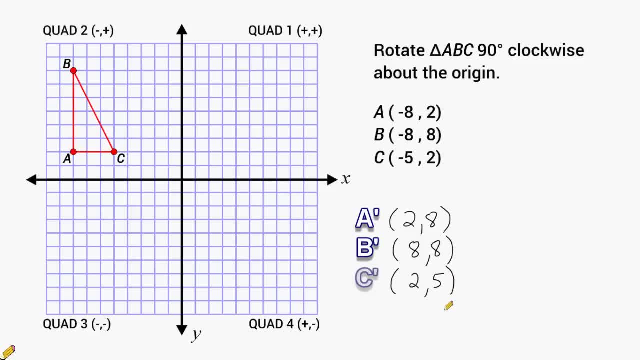 5 and once again, both the x and the y values will become positive because they are in quadrant number 1.. Now that we have the coordinates to where our triangle is going to be rotated to, let's go ahead and plot those points. 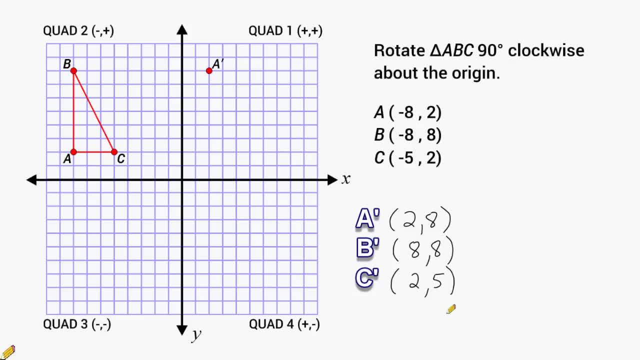 So point A is going to be at positive 2, positive 8 and point B is going to be at positive 8, positive 8.. And point C is at positive 2, positive 5.. So if we rotate our shape 90 degrees clockwise, you can see that our triangle will line up. 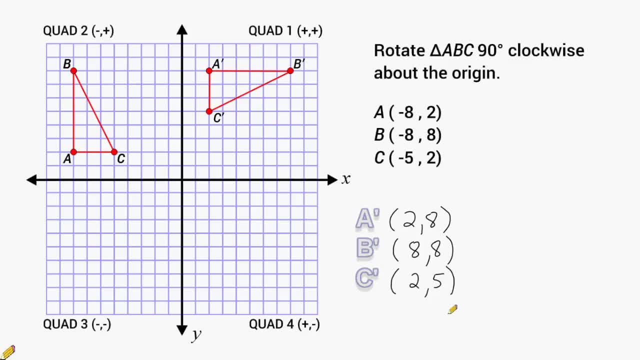 perfectly with the three points that we just plotted. Okay, let's take the original triangle that was located in quadrant 2 and rotate it 90 degrees counterclockwise around the origin. If you take a look at the arrow in the screen, you can see what direction counterclockwise. 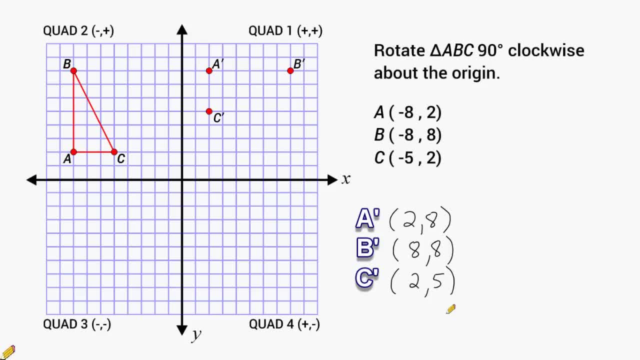 And point C is at positive two positive five. So if we rotate our shape ninety degrees clockwise, you can see that our triangle will look like this And it will line up perfectly with the three points that we just plotted. Okay, let's take the original triangle that was located in quadrant two. 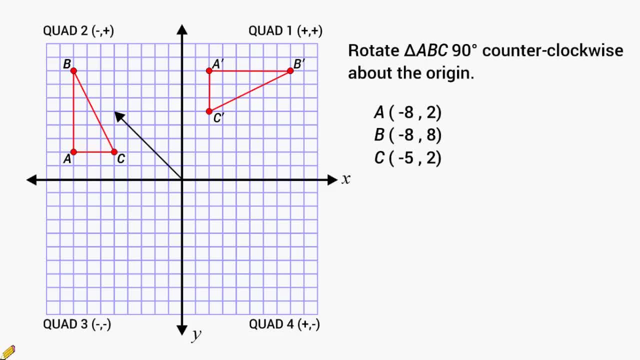 and rotate it ninety degrees counterclockwise around the origin. If you take a look at the arrow in the screen, you can see what direction counterclockwise is. So we are going to be rotating our triangle from quadrant two to quadrant number three. 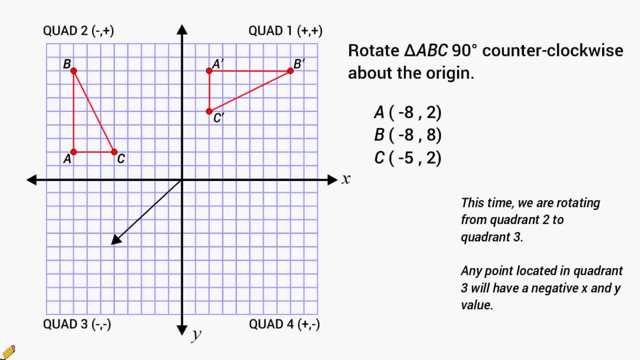 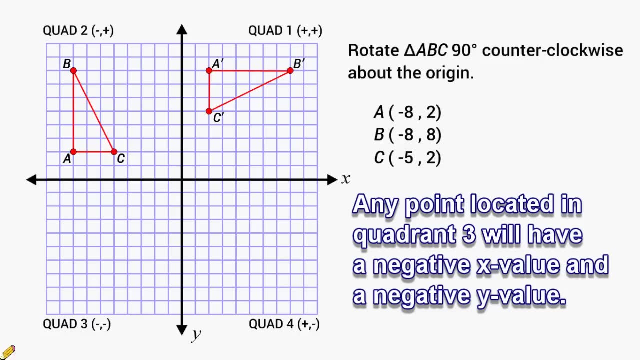 Now, the original points located in quadrant two had a negative x value and a positive y value. When rotating to quadrant number three, any point located within that quadrant will have a negative x and a negative y value. Okay, first, with any ninety degree rotation, remember we just switch around the absolute values of our x and our y value. 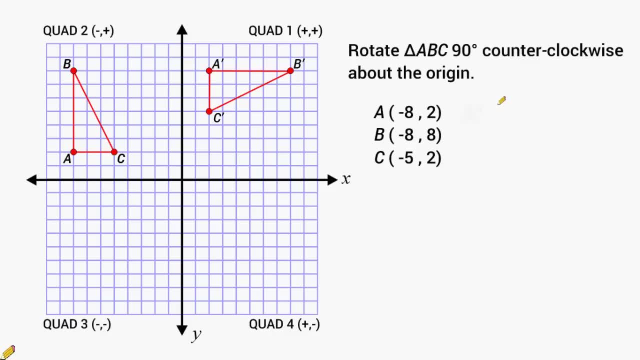 So our point was at negative eight and positive two. So we take those absolute values and switch them around to be two and eight And because this point is located in quadrant number three, we have to make sure that both the x and the y value is negative. 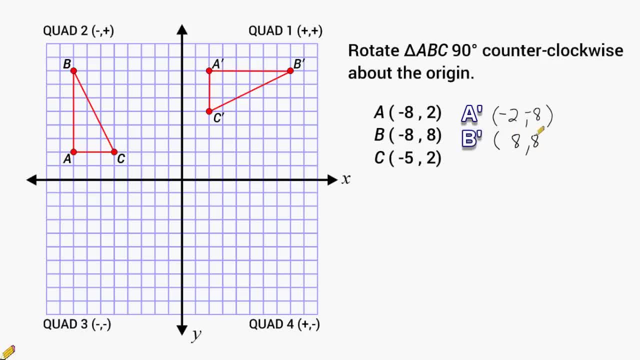 And with point B both of the absolute values were eight. So we just write two eights. but we have to make them both negative And the original location of point C was negative five and positive two. So we just go ahead and switch those two numbers. 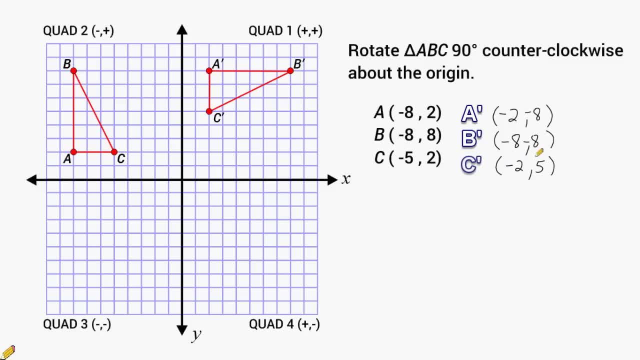 and make sure that they are both negative, because they are in quadrant number three. Okay, after you have found the location to where your shape is going to be rotated to you, just go ahead and plot those points and then you can form your shape connecting those points together. 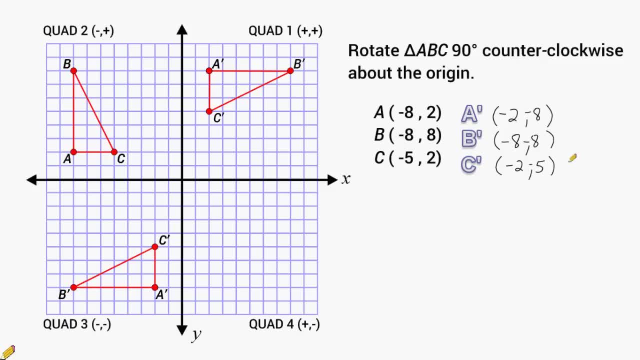 And that will be the location of your rotated object. Now, another way to look at a ninety degree rotation is by considering the x and the y axis itself being rotated. Notice: if we rotate our x and our y axis, the original location of point A, along with the origin. 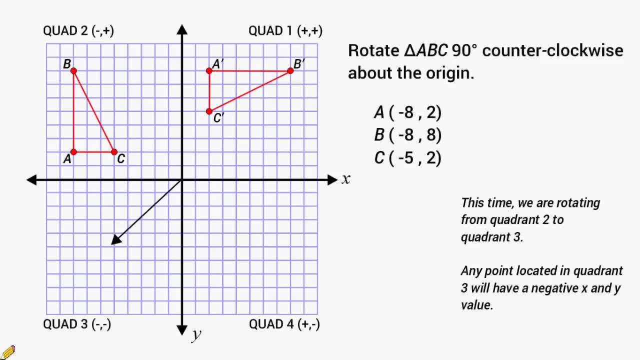 is So. we are going to be rotating our triangle from quadrant 2. To quadrant number 3.. Now, the original points located in quadrant 2 had a negative x value and a positive y value, And when rotating to quadrant number 3, any point located within that quadrant will have. 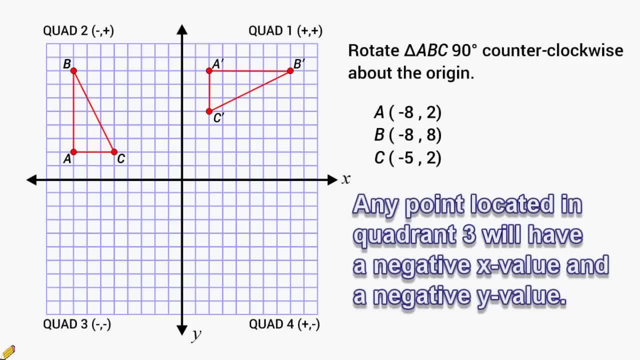 a negative x and a negative y value. Okay, first, with any 90 degree rotation, remember, we just switch around the absolute values of our x and our y value. So our point was at negative 8 and positive 2. So we take those absolute values and switch them around. 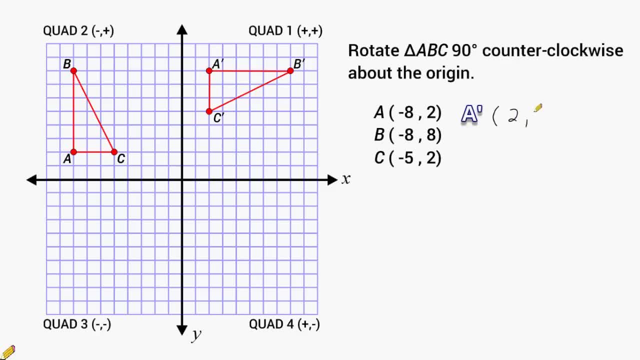 Okay, let's go ahead and plot those points. We can switch them around to be 2 and 8. And because this point is located in quadrant number 3, we have to make sure that both the x and the y value is negative. 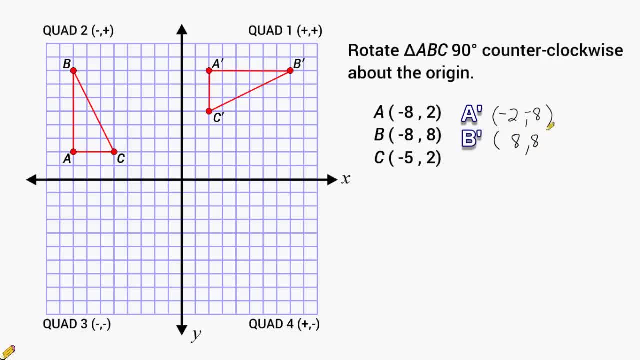 And with point B both of the absolute values were 8. so we just write two 8's, but we have to make them both negative And the original location of point C was negative 5 and positive 2.. Okay, So we just go ahead and switch those two numbers. 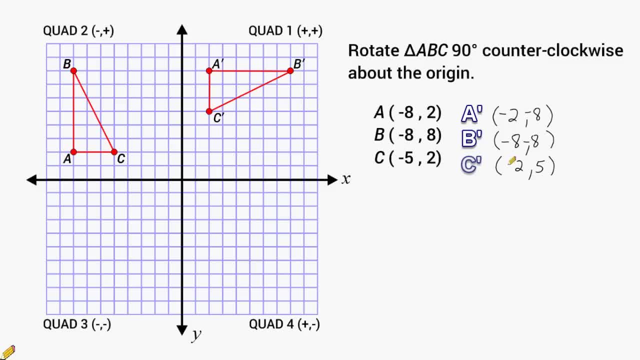 and make sure that they are both negative, because they are in quadrant number three. Okay, after you have found the location to where your shape is going to be rotated to you, just go ahead and plot those points and then you can form your shape connecting those points together. 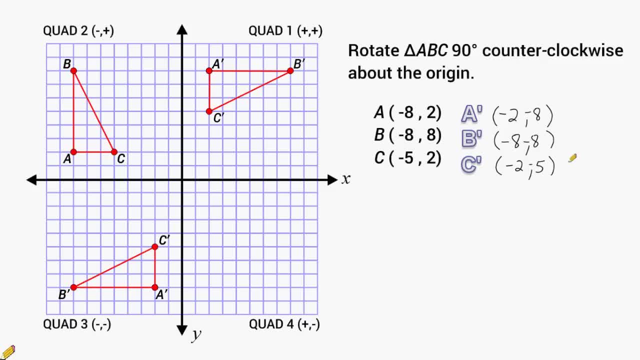 And that will be the location of your rotated object. All right now, another way to look at a 90 degree rotation is by considering the X and the Y axis itself being rotated. Notice: if we rotate our X and our Y axis, the original location of point A, along with the origin. 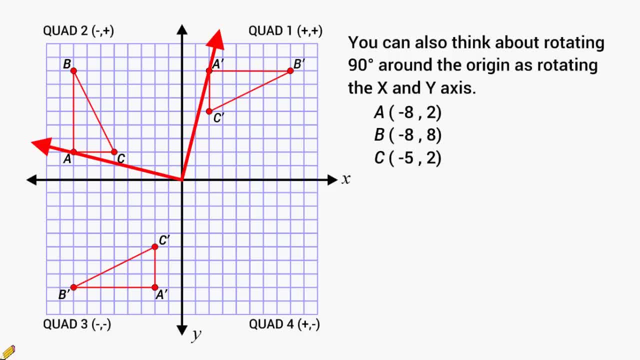 along with the new location of point A, will form a right angle. And if we continue our rotation clockwise, both points C's, along with the origin, will form a right angle, and also the original location of point B will form a right angle, The new location of point B. 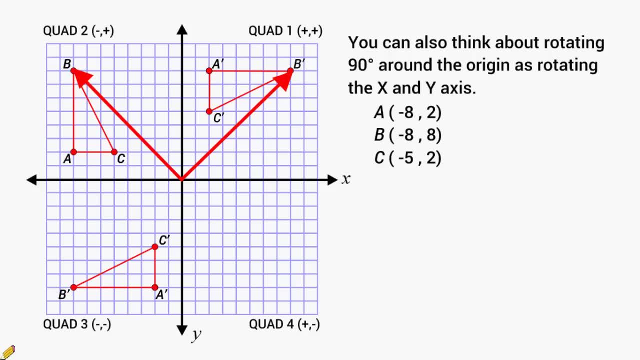 and the origin form a right angle And then, if we continue our rotation clockwise, notice that where the Y axis was is now lined up with the X axis, and where the X axis was is now lined up with the Y axis, And this is why we can simply switch around.